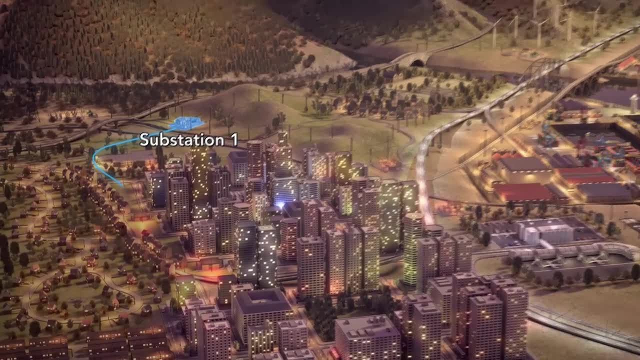 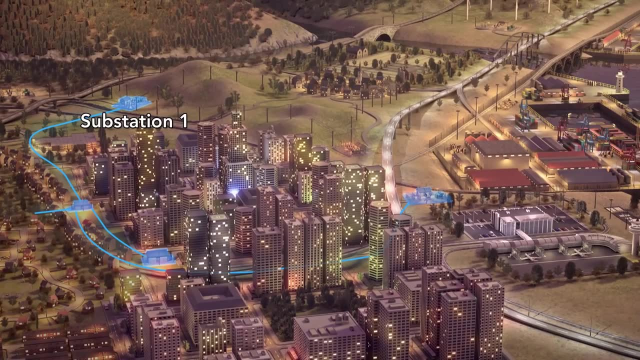 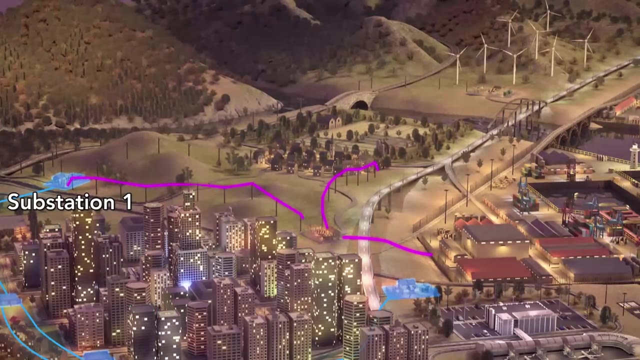 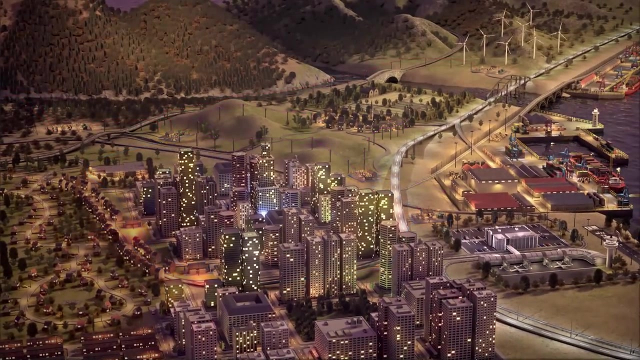 The primary substation provides a feed-out to a residential area, a commercial city district and the local airport via other local substations. A busy port and a small rural community are also supplied by the primary substation through another. Let's see how the SCADA system is used to manage and maintain the network during a fault. 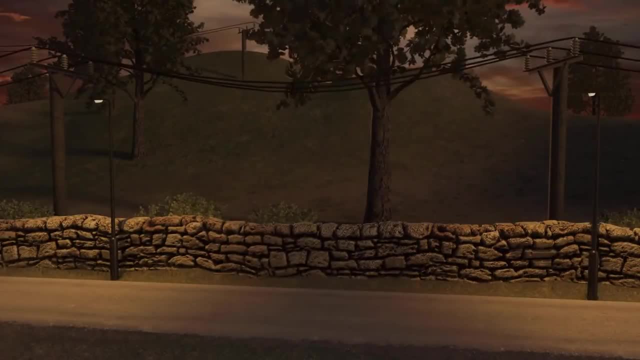 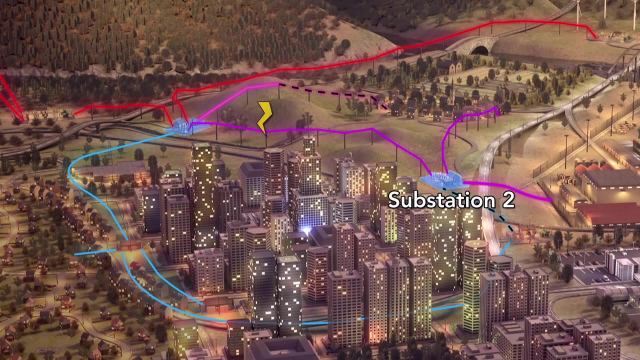 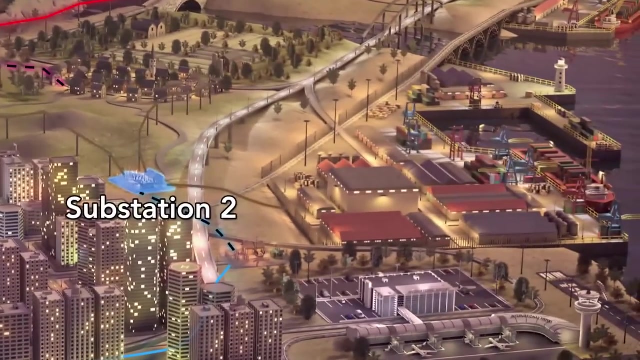 On a remote rural section of the network, a fallen branch causes damage to the overhead power lines feeding substation 2.. This break in supply causes the circuit breaker for this line to trip at the primary substation, leading to a total power outage to both the port. 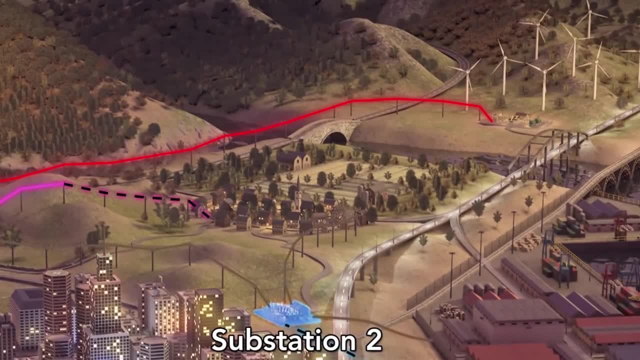 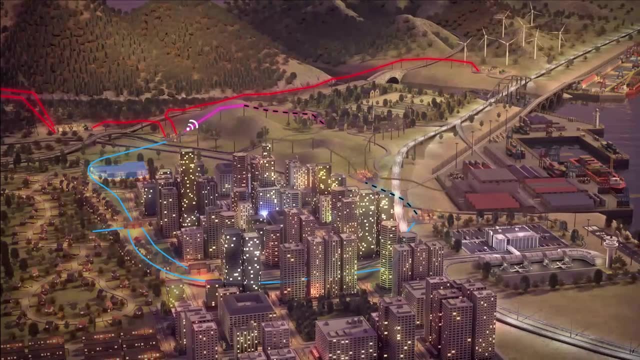 and the rural community that runs the SCADA system. This means that the SCADA system will not rely on this circuit. Power to the rest of the network remains unaffected. The SCADA system receives notification of the circuit breaker trip, then uses the fault passage indicators positioned around the network to determine where the fault has occurred. 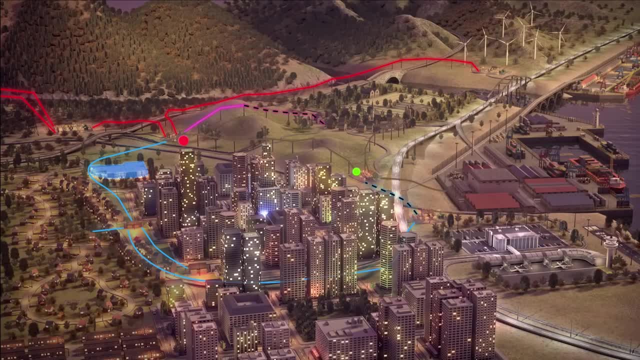 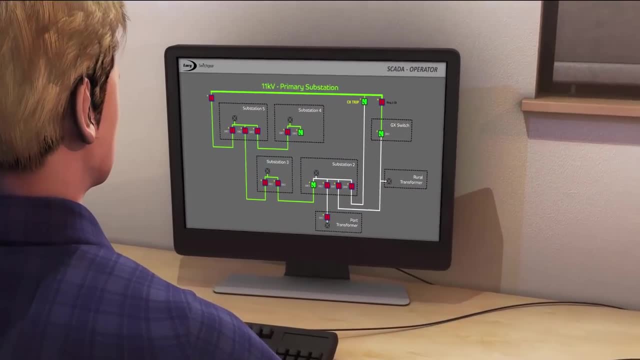 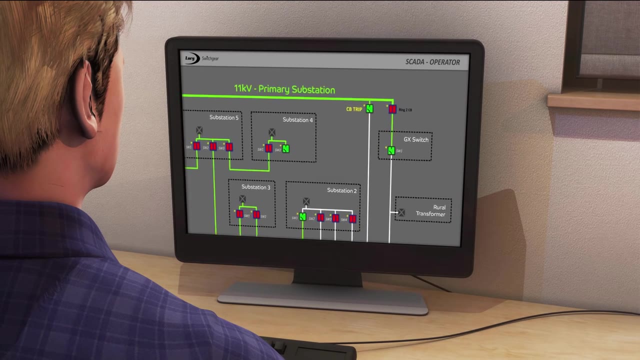 In this case the fault passage indicator at substation 2 has not tripped, so at the remote SCADA data center the operator is informed that the fault must be somewhere on the line between the primary substation and substation number 2.. The operator can now use the Lucy Switchgear SCADA system to isolate this area and re-route power to customers without a supply. 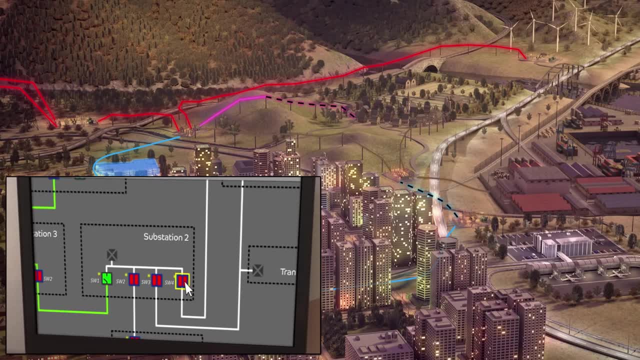 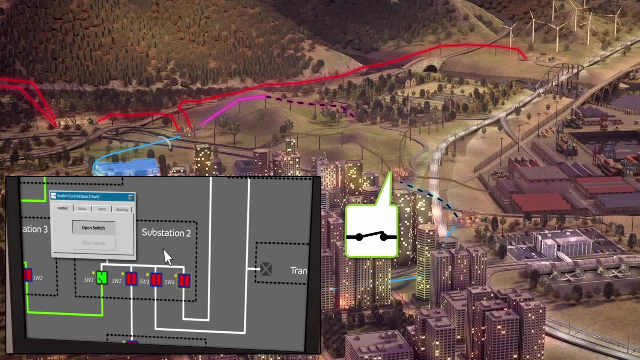 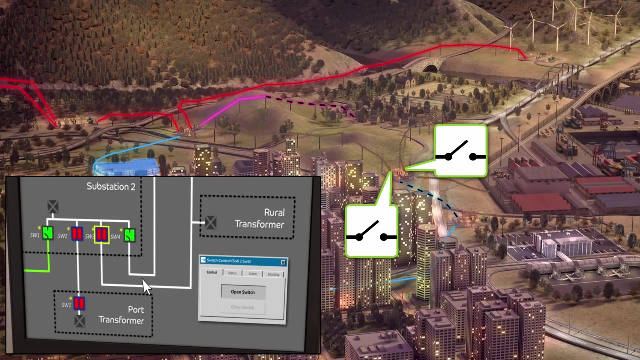 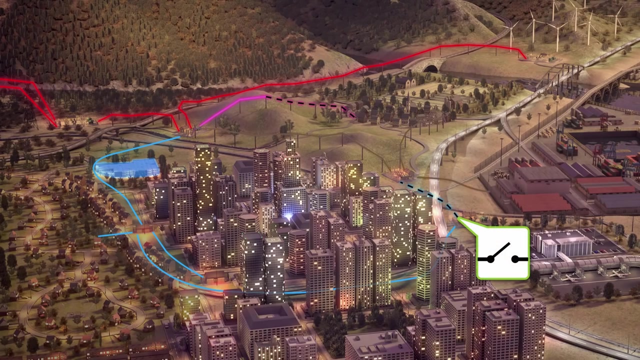 The operator remotely opens the incoming switch from the primary substation to substation 2 and then opens the outgoing switch from substation 2 to the rural community. This totally isolates the fault area from the rest of the network. The operator can now close the outgoing switch at substation 3 to re-energise the link to substation 2.. 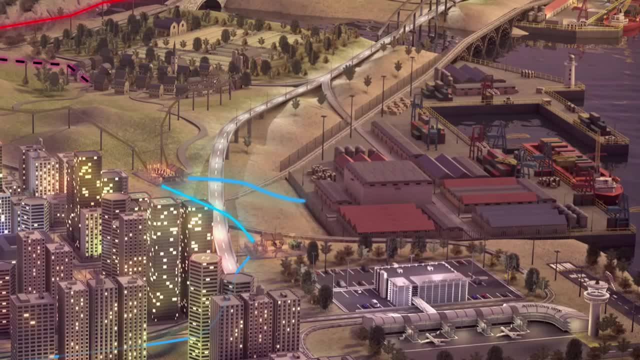 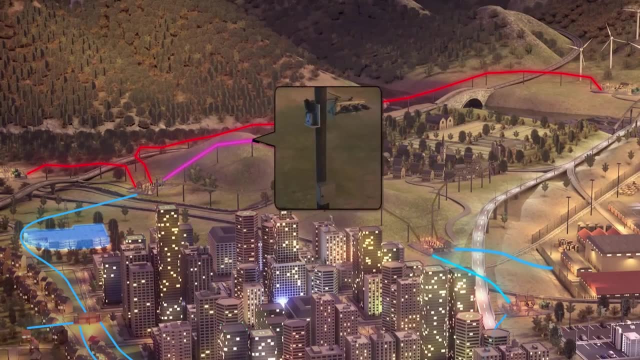 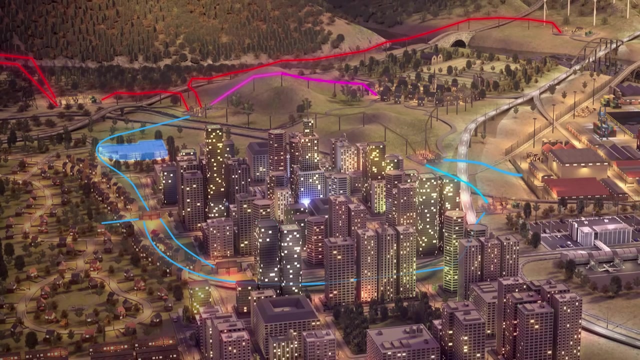 Substation 2 can now reinstate the supply to the port In order to avoid overloading one side of the network, the operator chooses instead to close the GX switch on the backfeed to the rural community to reinstate their supply. Supplies to all affected areas are now complete and the faulty line is safely isolated from the network.